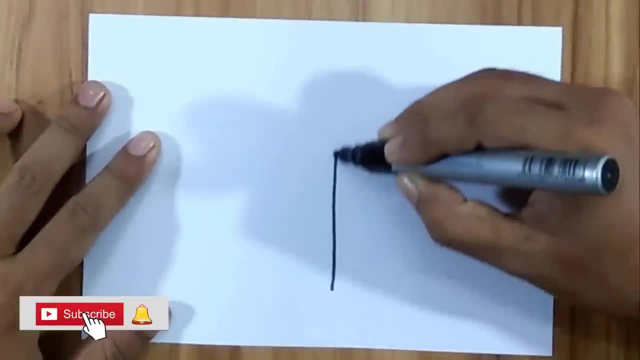 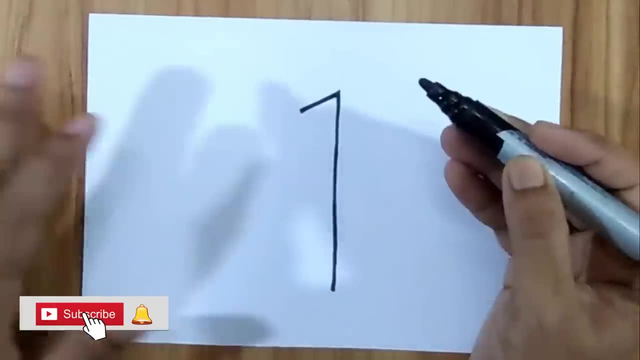 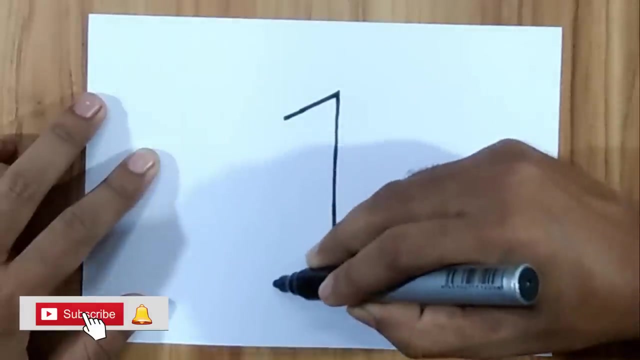 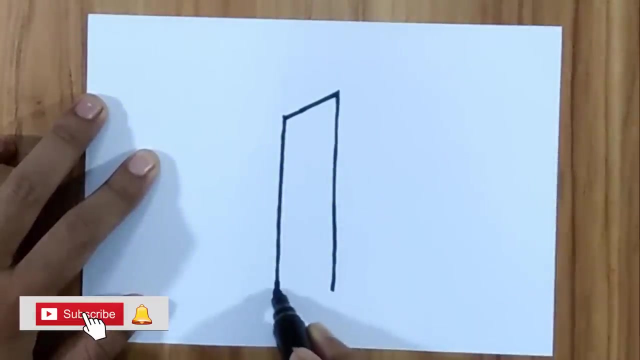 A tisket, a tasket, a green and yellow basket. I wrote a letter to my love. and on the way I dropped it, Dropped it, I dropped it. and on the way I dropped it, A little boy. he picked it up and put it in his pocket. 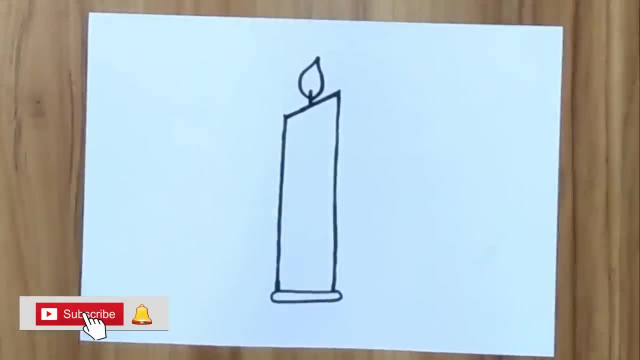 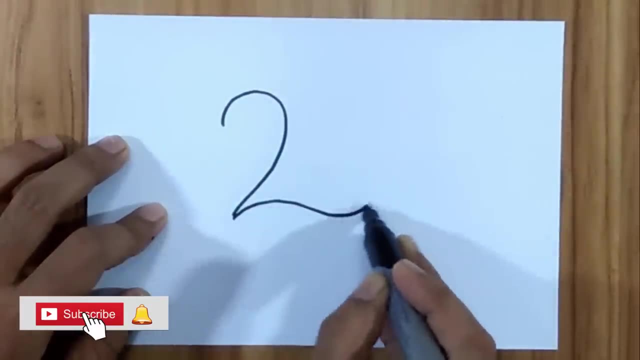 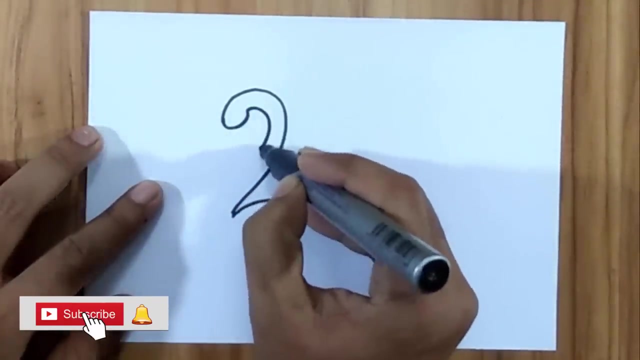 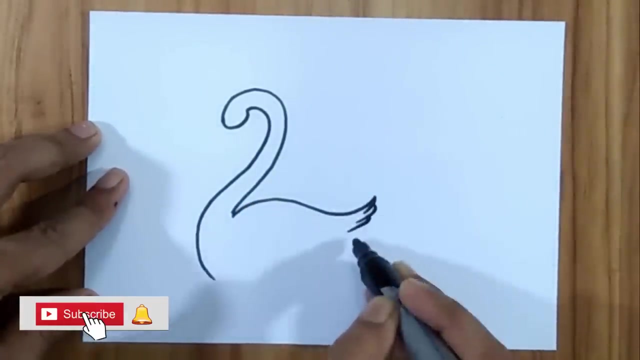 A tisket, a tasket, a green and yellow basket. I wrote a letter to my love. and on the way I dropped it, Dropped it, I dropped it. and on the way I dropped it, A little boy. he picked it up and put it in his pocket. 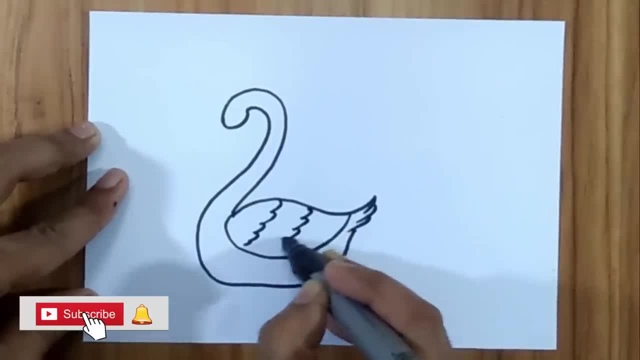 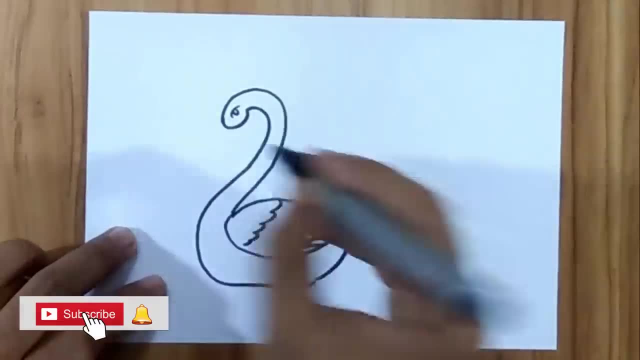 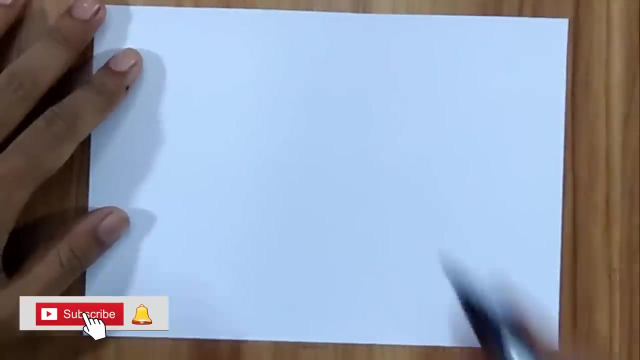 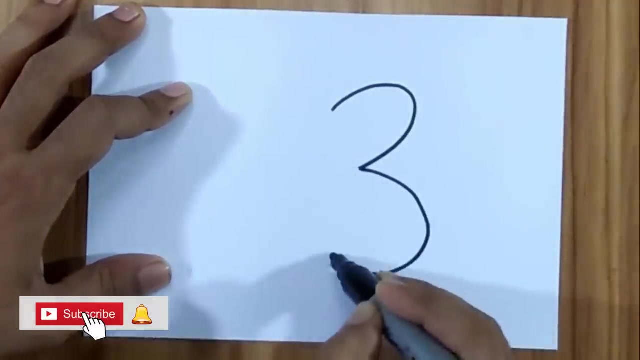 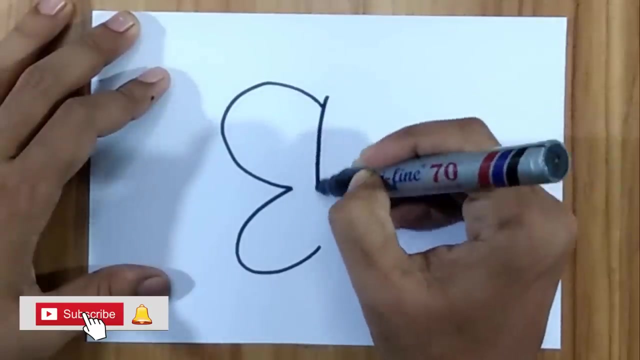 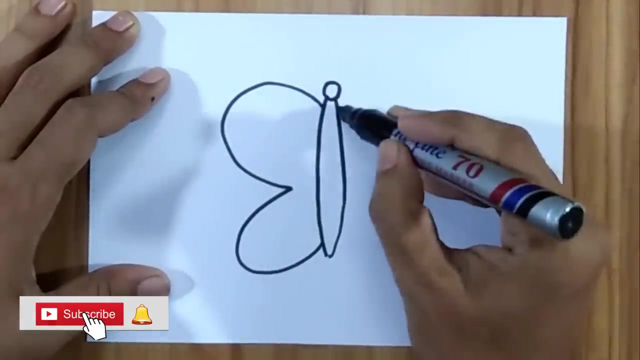 A tisket, a tasket, a green and yellow basket. I wrote a letter to my love. and on the way I dropped it, Dropped it, I dropped it. and on the way I dropped it, A little boy. he picked it up and put it in his pocket. 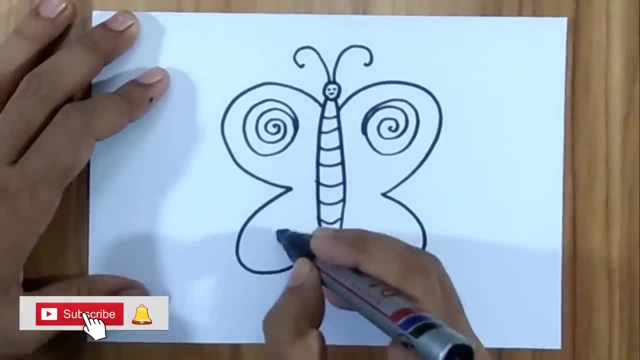 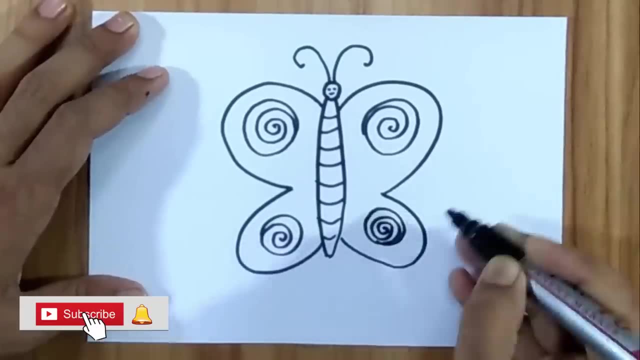 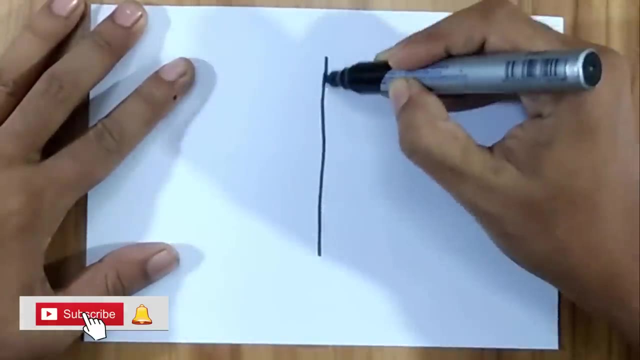 A tisket, a tasket, a green and yellow basket. I wrote a letter to my love and on the way I dropped it, On the way I dropped it, On the way I dropped it, Put it in his pocket. Put it in his pocket. 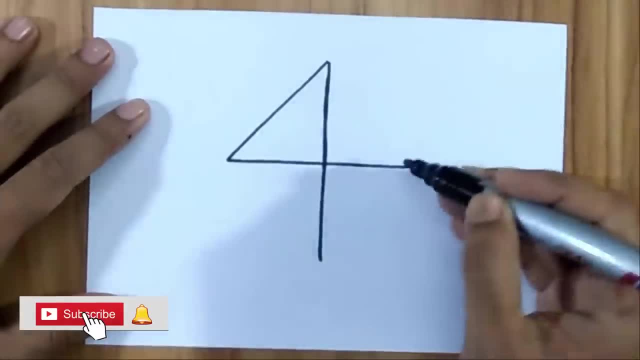 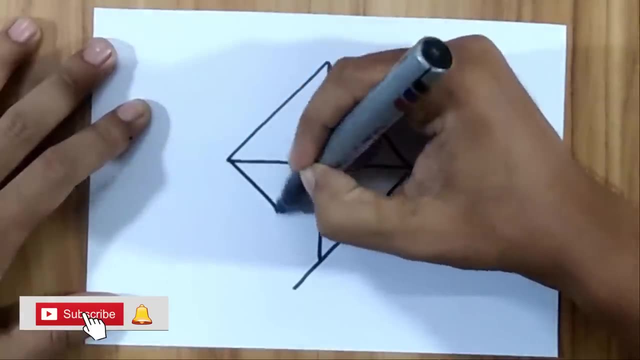 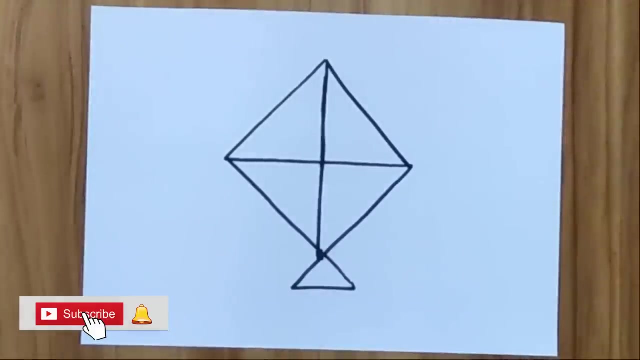 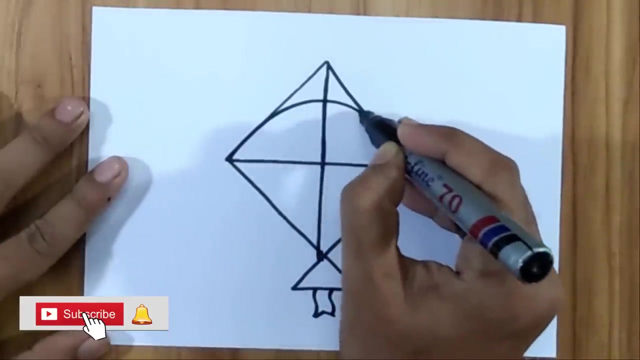 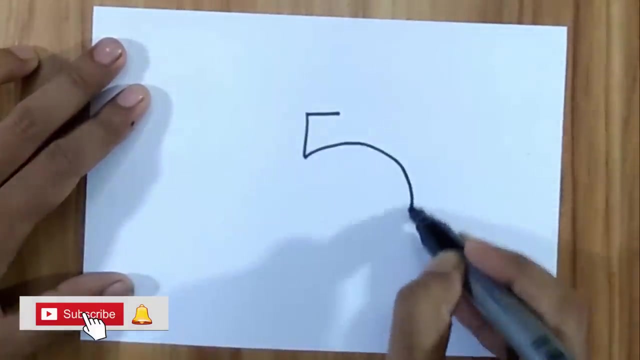 On the way I dropped it. On the way I dropped it: A disket, a tasket, a green and yellow basket. I wrote a letter to my love. and on the way I dropped it, Dropped it, I dropped it. and on the way I dropped it, 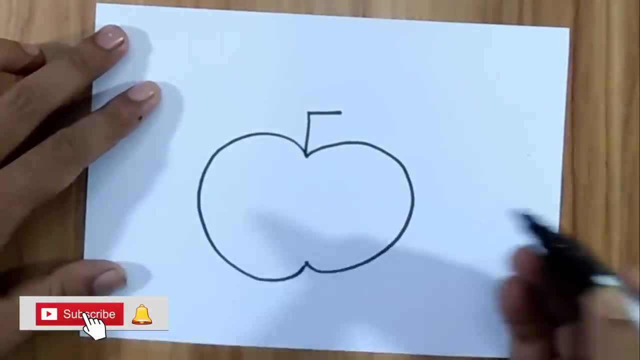 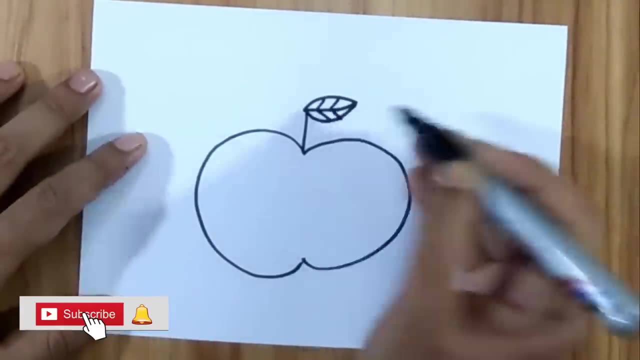 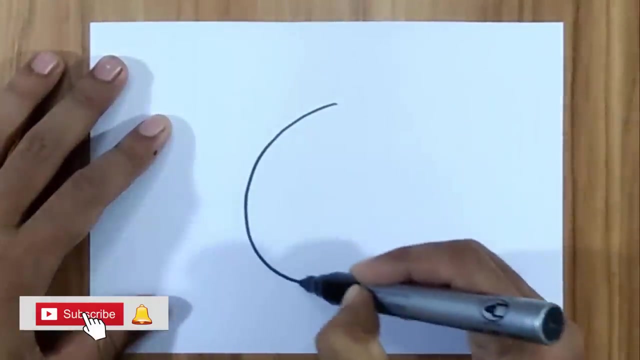 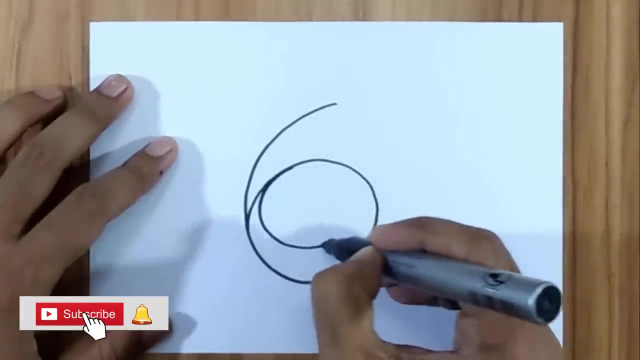 A little boy. he picked it up and put it in his pocket: A disket, a tasket, a green and yellow basket. I wrote a letter to my love. and on the way I dropped it, Dropped it, I dropped it. and on the way I dropped it. 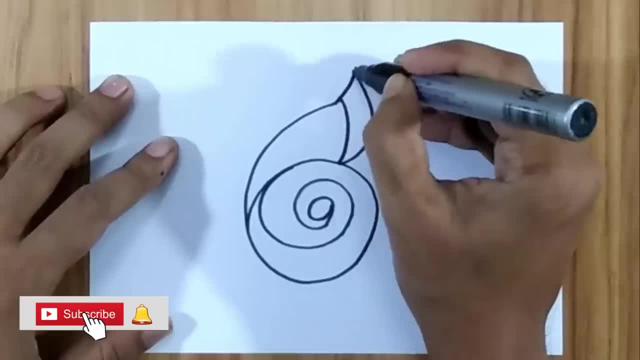 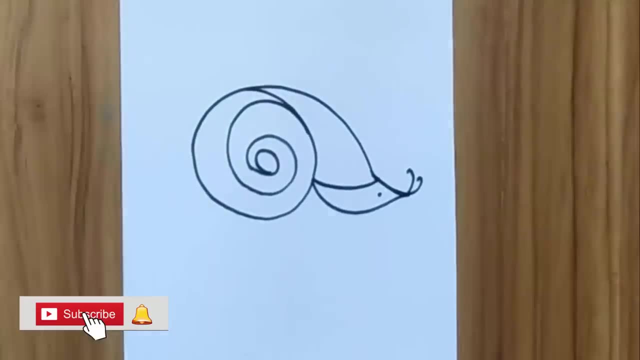 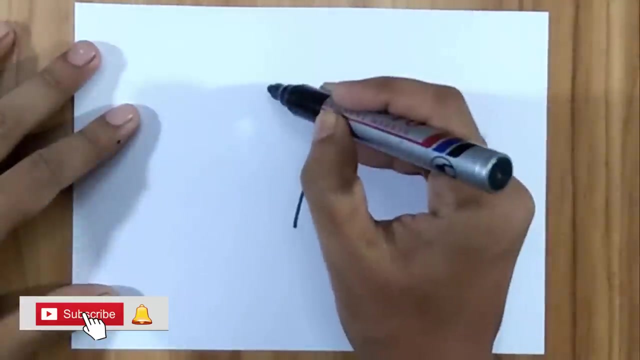 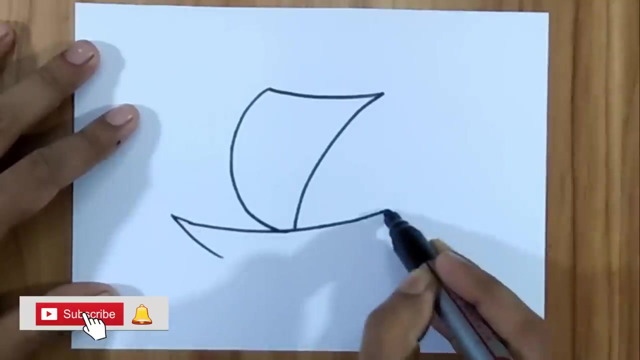 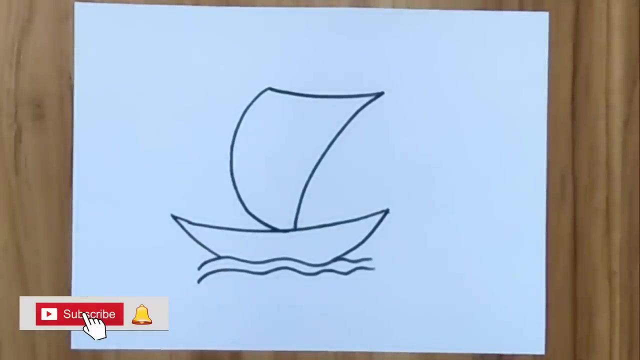 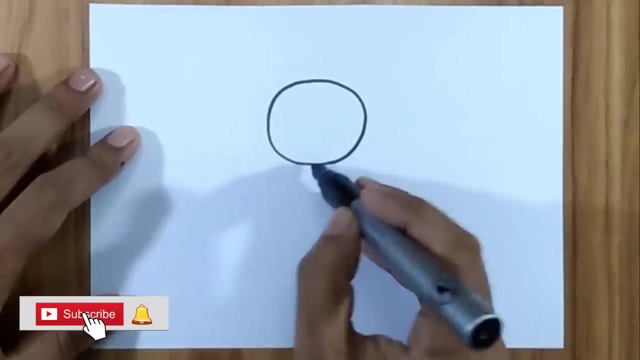 A little boy. he picked it up and put it in his pocket: A disket, a tasket, a green and yellow basket. I wrote a letter to my love. and on the way I dropped it, Dropped it, I dropped it. and on the way I dropped it. 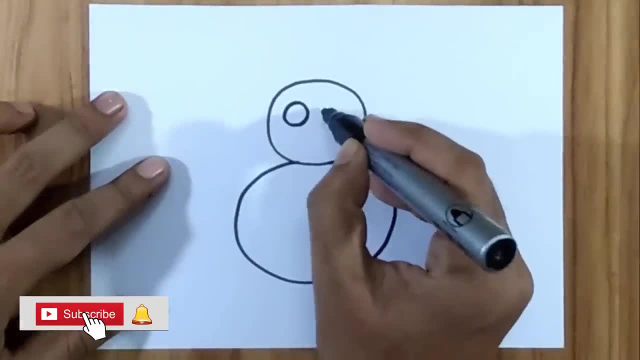 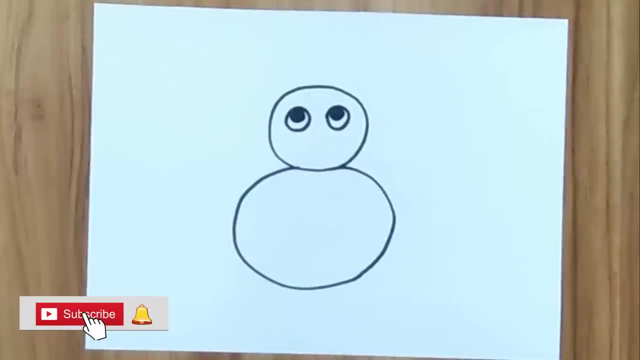 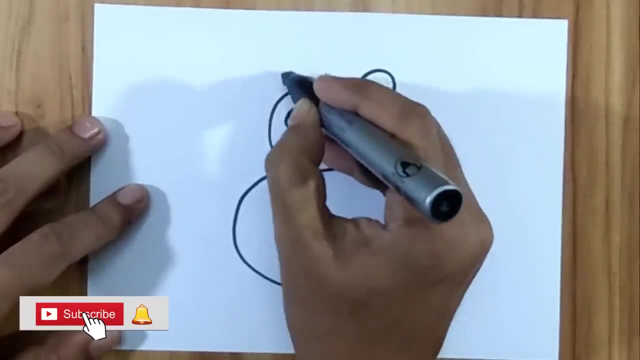 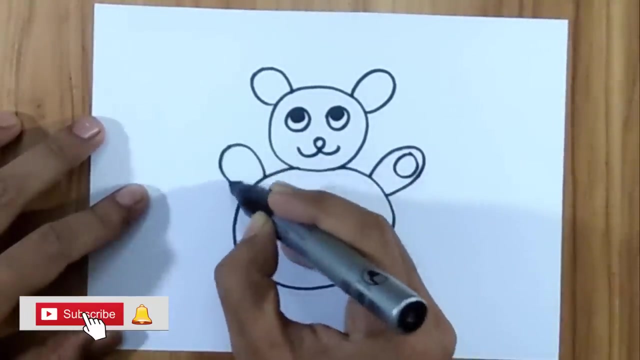 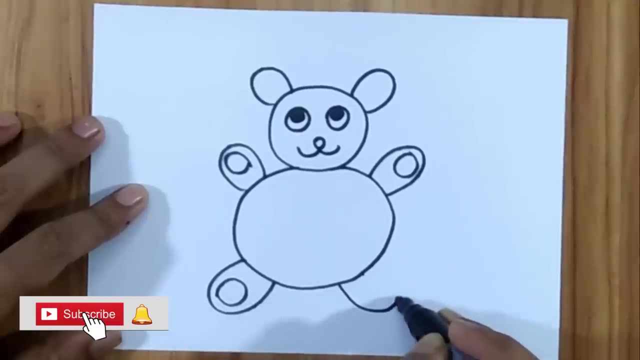 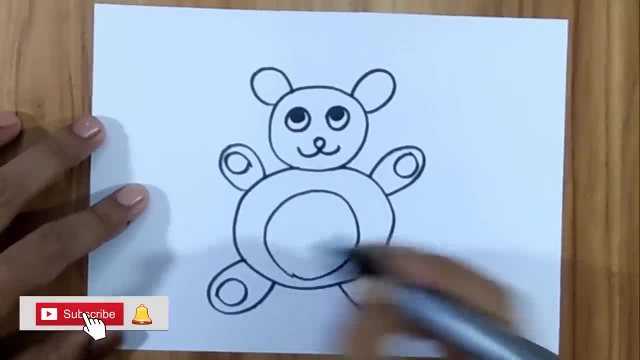 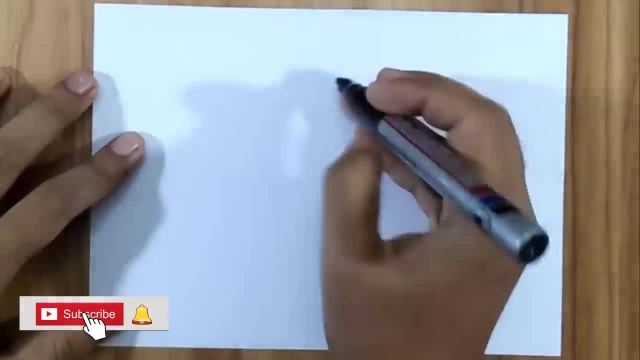 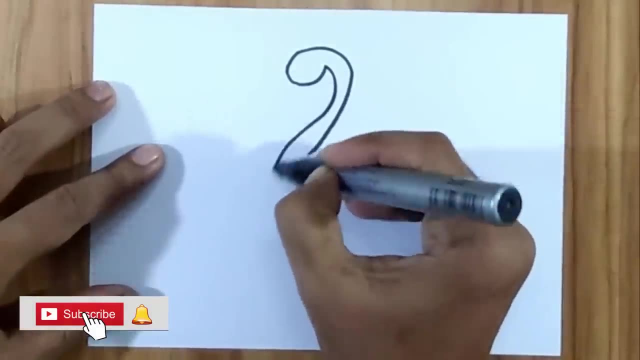 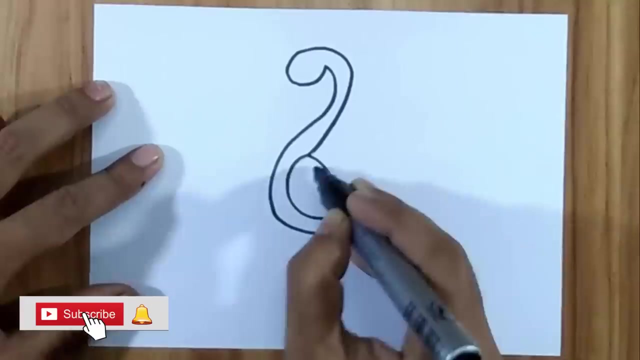 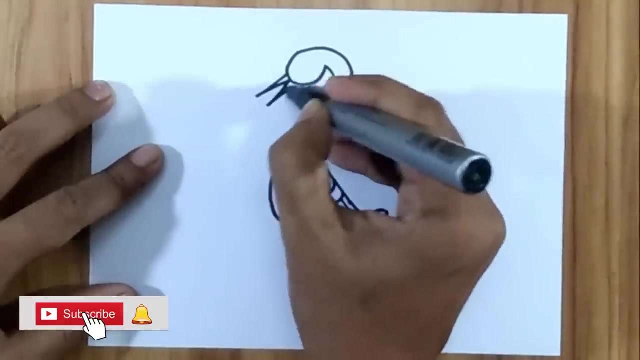 Dropped it, I dropped it. and on the way I dropped it, Dropped it, I dropped it and on the way I dropped it, Put it in his pocket. On the way I dropped it. On the way I dropped it. A-tisket, a-tasket- a green and yellow basket.